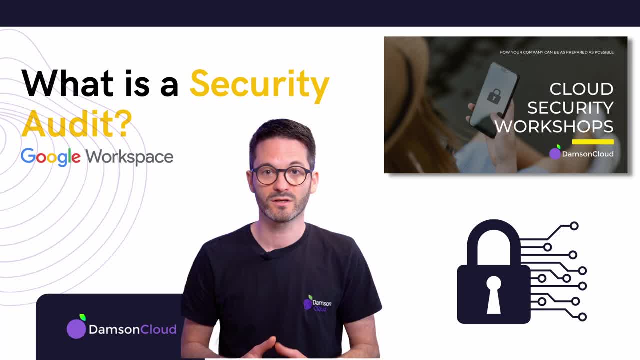 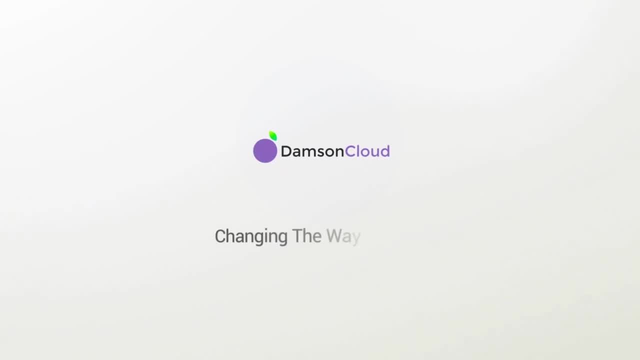 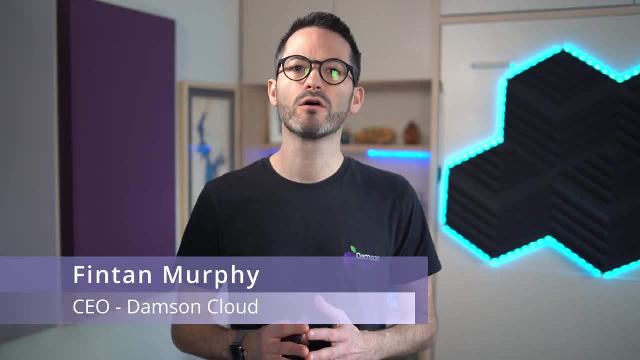 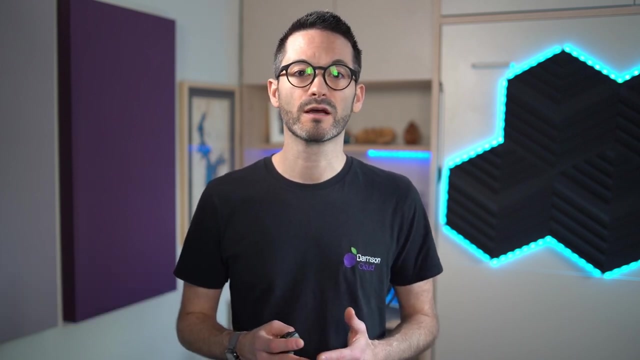 Hi everybody, Fintan here from Damson Cloud, and this week I wanted to talk about security audits. They're a popular service here at Damson Cloud and I thought it might be valuable to run through exactly what they are. I'm going to cover what is a security audit, why you should get. 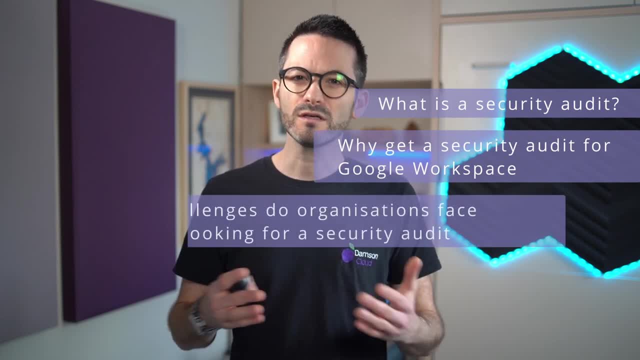 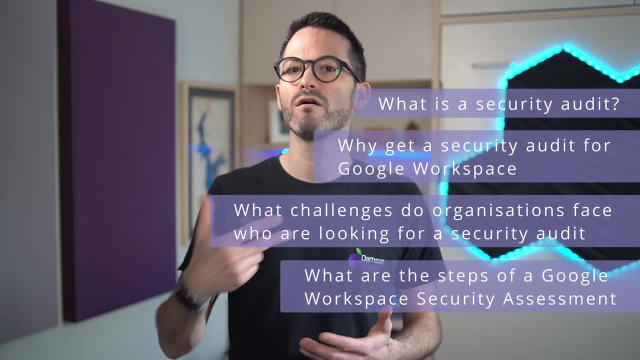 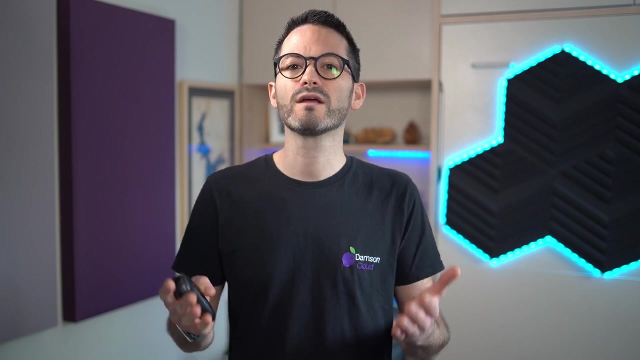 a security audit for your Google Workspace environment. what kind of challenges do organisations face, who are looking for security audits and, finally, what are the steps of a Google Workspace security assessment or audit that we actually take when we take you through them? So, firstly, what is a security audit? Well, the Google Workspace security assessment or audit. 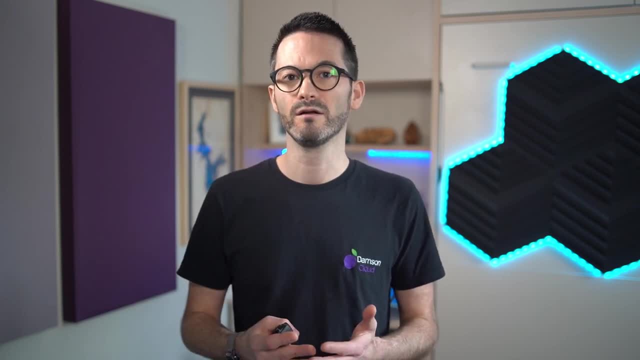 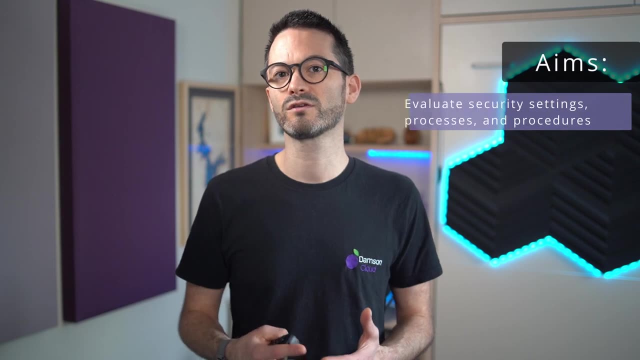 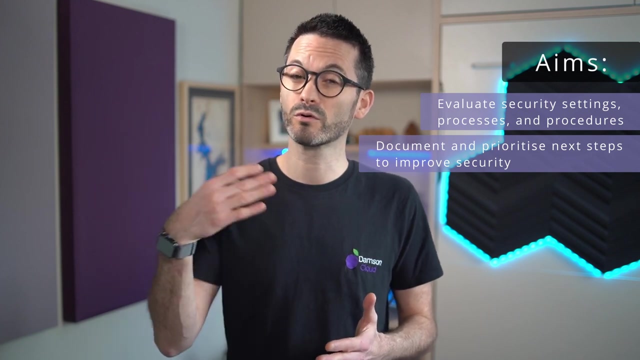 helps improve the security posture of your Google domain through an assessment of the current configurations, security processes and procedures. It aims to evaluate the security settings and processes and procedures, document and prioritise the next steps to help you actually improve your security posture and also train. 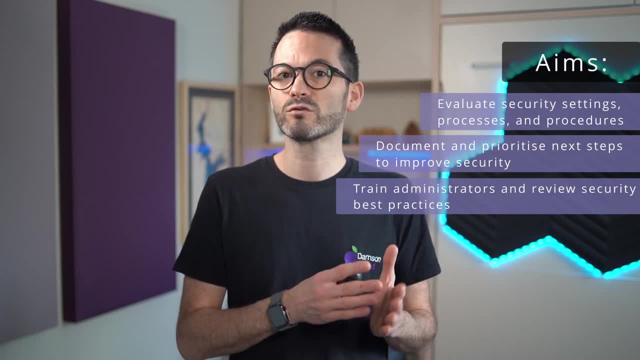 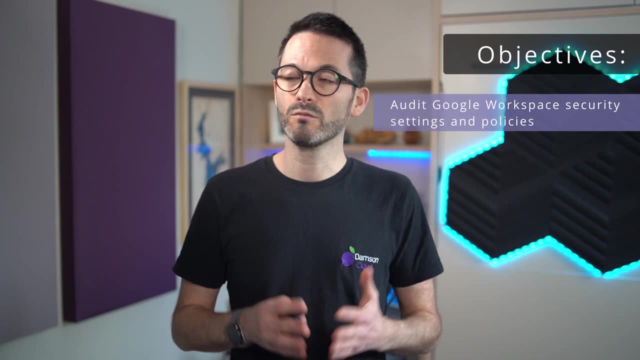 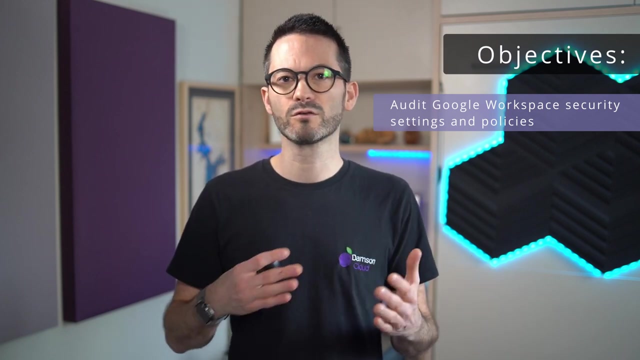 your administrators and IT team on how to review the security best practices. There's a couple of objectives here: obviously, auditing the Google Workspace settings, and we find that customers they haven't often done that, you know. maybe it was something that they did when they first moved to Google, but it's not something. 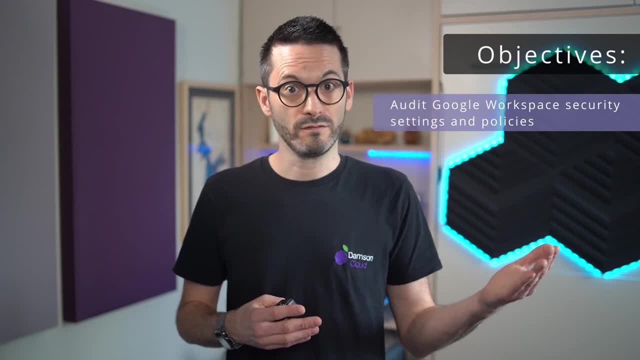 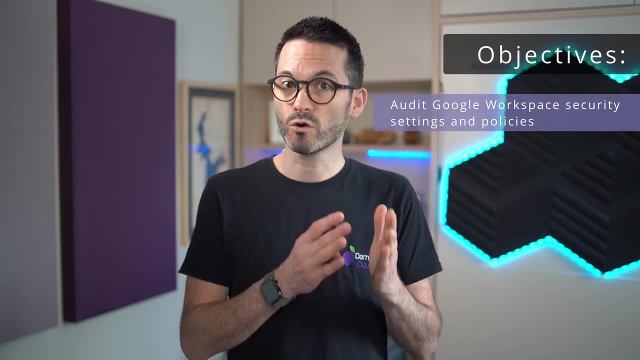 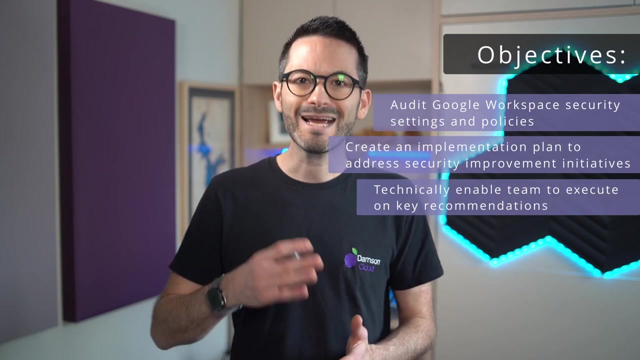 that they're kind of doing on a regular basis. maybe it's been a few years or even longer, and they just really want to document those and write them down so that they have that recorded somewhere. Create an implementation plan to address the security improvements and initiatives and technically enable your team to execute on these key recommendations. 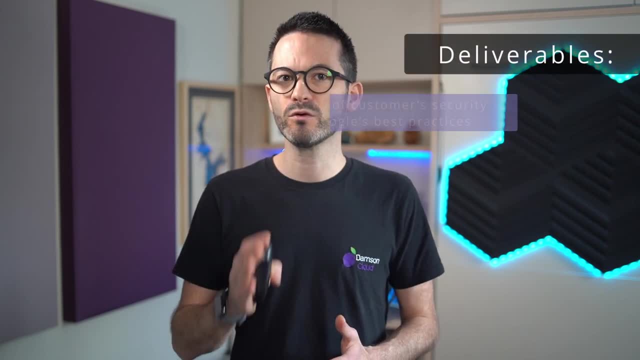 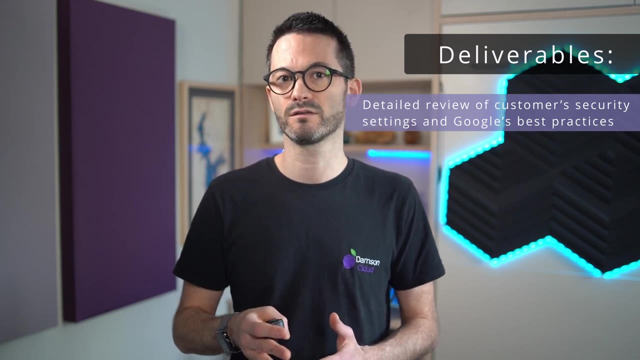 There's a couple of deliverables as well. we will give you a document that will give you a detailed review of your actual security system. So, if you're looking for a security system that's based on the security settings, Google's best practices, an executive review of the recommendations. 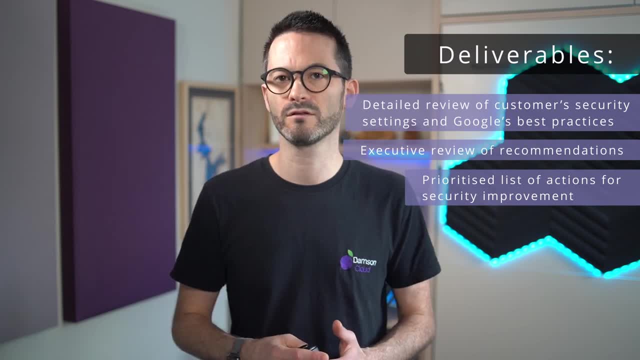 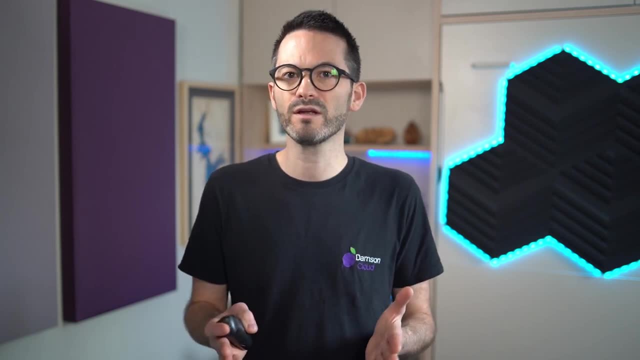 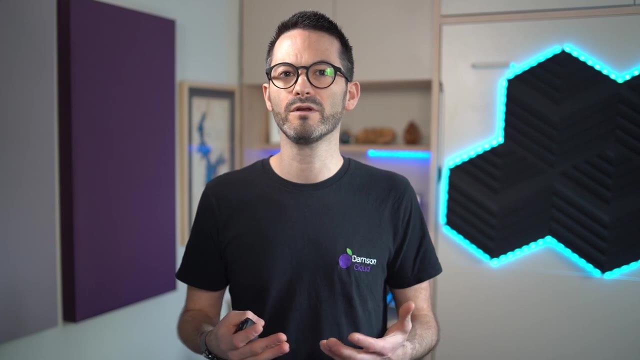 and a prioritised list of the actions that we recommend that you should take. So why would you get a security audit? Well, there are many reasons why organisations want to get a security audit of their Google environment. However, there are kind of a couple of common. 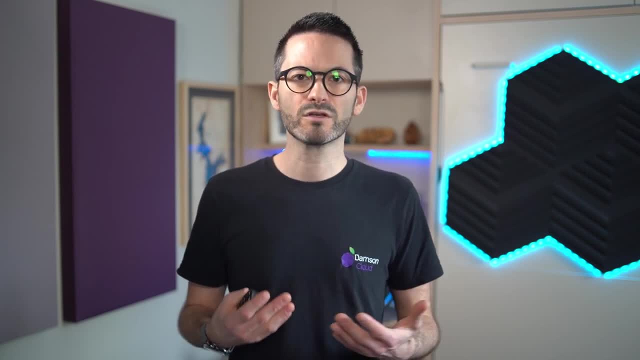 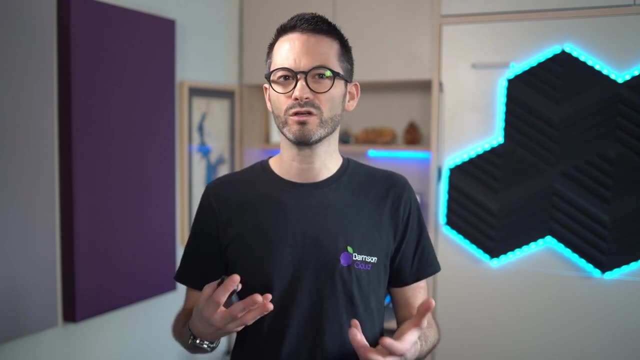 reasons that people tend to come to us- I'd say probably the top three- are around eliminating risks. they want to guard against new and existing security threats and they want to make sure that they're kind of leveraging all of the tools that are at their disposal already. Awareness is another. 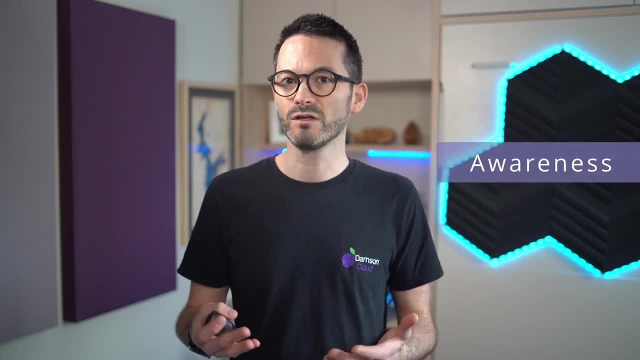 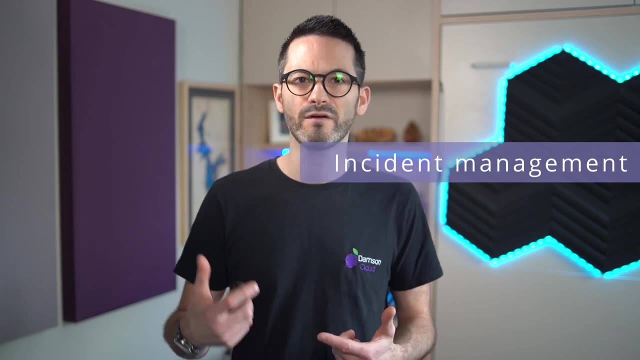 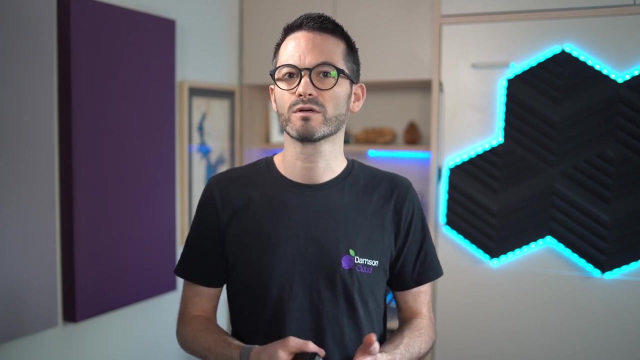 big one, where they want to improve and adopt the security features amongst their IT team and indeed their end users. and then the other area tends to be incident response management, where they want to increase the effectiveness of actually responding to an incident if, or indeed when, it might occur within the organisation, particularly around Google Workspace. 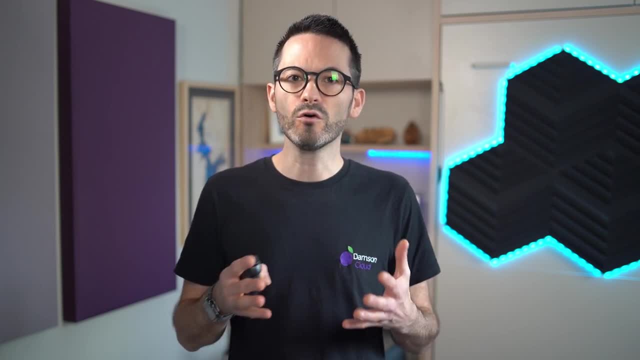 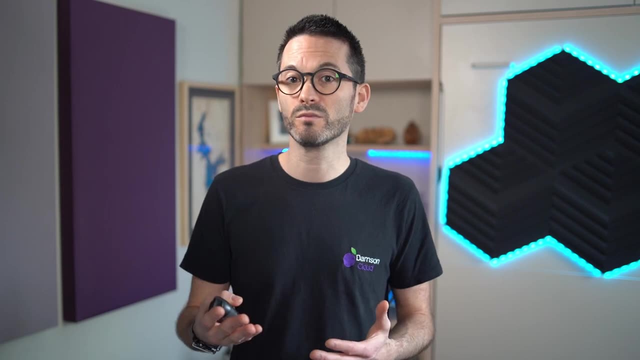 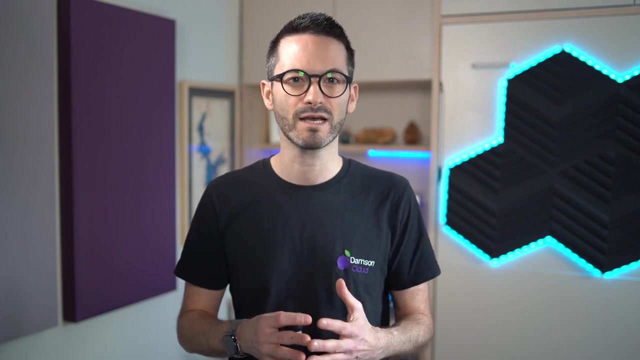 So what are the challenges that organisations tend to face? who are looking for a security audit? Well, often we're talking to the IT teams and they've perhaps taken over from somebody else, so they didn't actually set up the Google Workspace environment and they maybe feel that they can't kind of stand over the settings and the policies that are in. 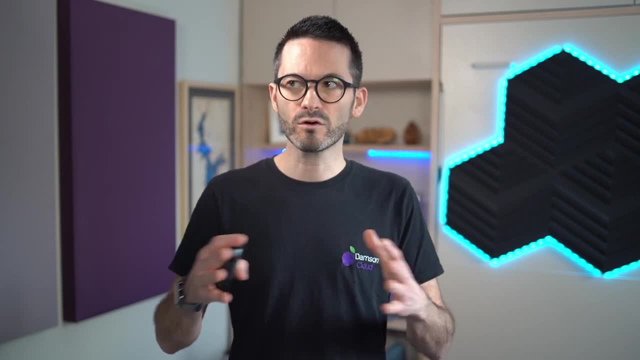 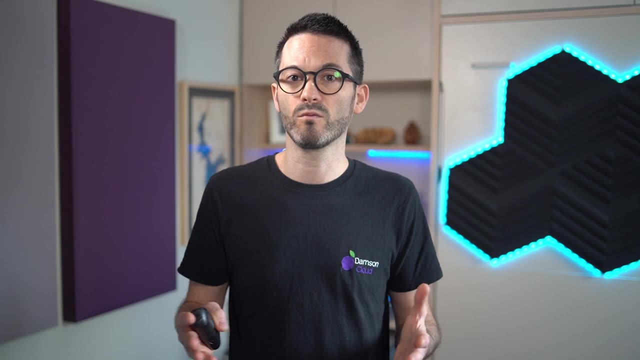 place, so they want someone else to come in as a third party and just look at those settings and say, yes, this is how we would set this up as a Google Partner who's done this hundreds of times is what we would recommend. and the other area is if an organization has grown very rapidly, maybe 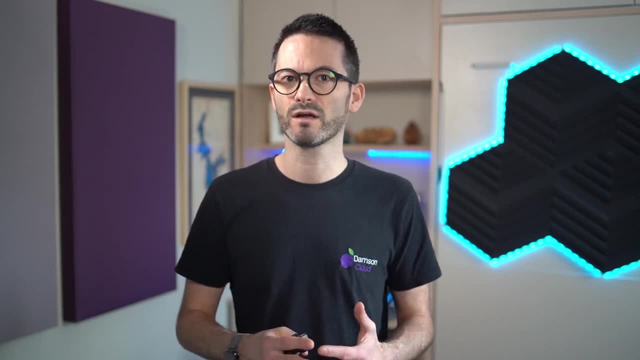 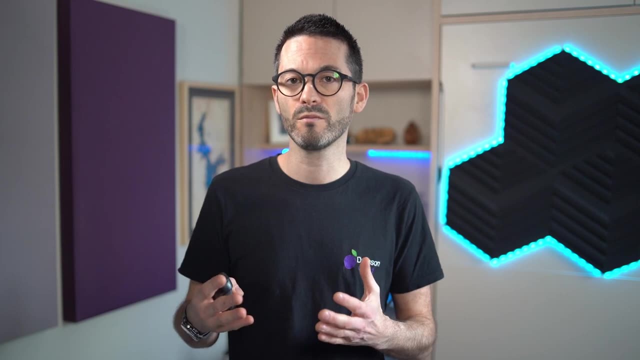 they've. they've had a lot of growth or they've gotten funding and they've grown very quickly and maybe the settings that they had in place in the organization was small, was fine, but now they need someone again to kind of come in and look and say: well, now we're 100 staff, now we're now. 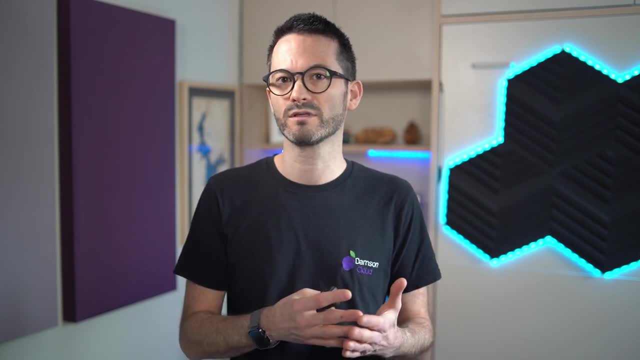 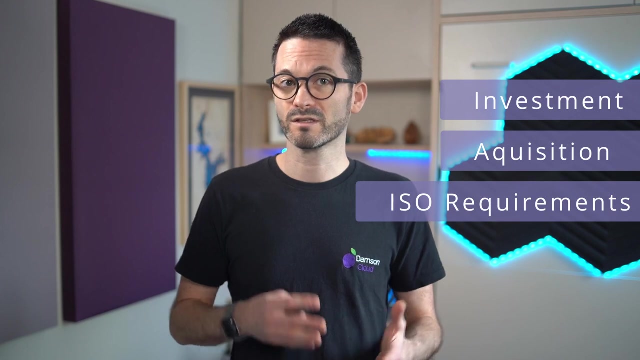 we're 500 staff and we have these other requirements now that we didn't have before. this can sometimes be accompanied by external factors. perhaps the organization wants to increase its security posture because of investment or acquisition, or indeed an iso um requirement. that's that's often. 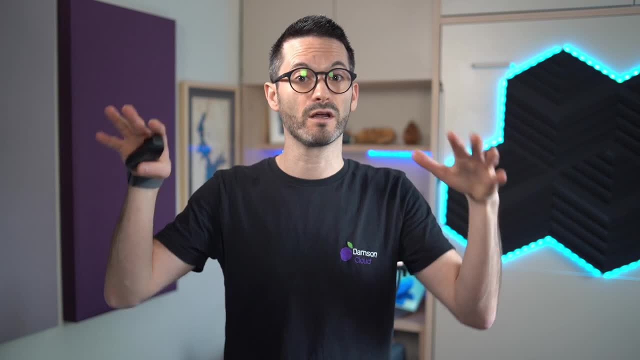 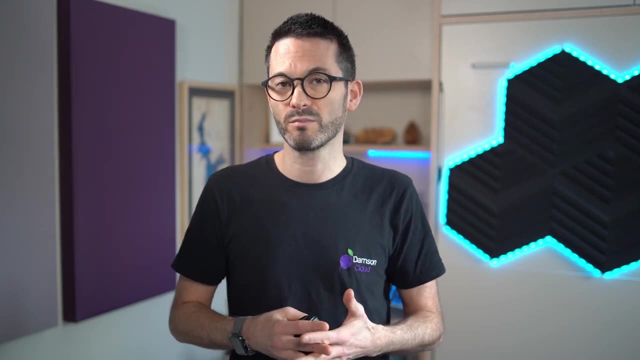 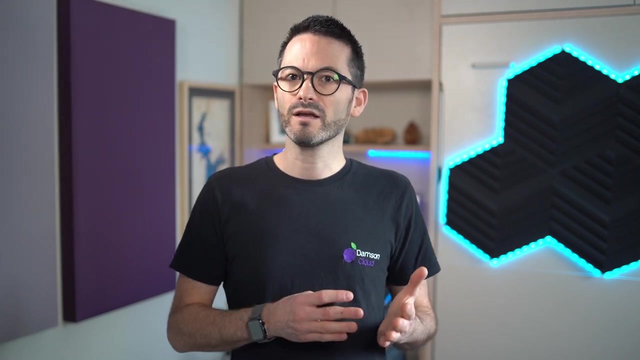 you know, customers may be doing an iso certification. at another level, they're looking at all of their it systems and google workspace obviously being one of the core systems that our business is using and that all of their users are using and will fall under that as well. and the other area is if 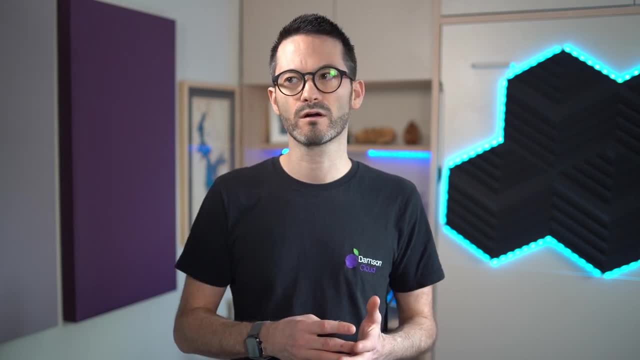 a customer has upgraded to a higher tier. so we see this where customers upgraded to, maybe, enterprise from one of the business tiers and again they don't feel like they're fully leveraging all of the security features on the platform. and this again is common when an organization is is growing. 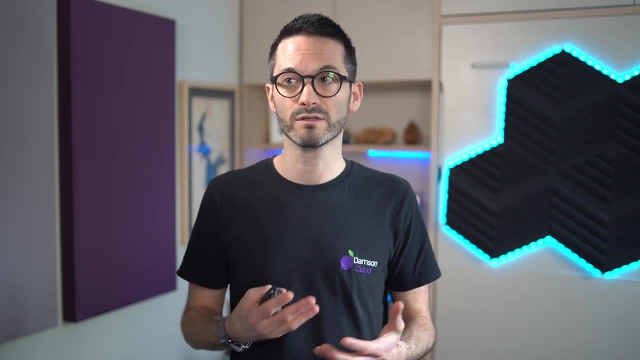 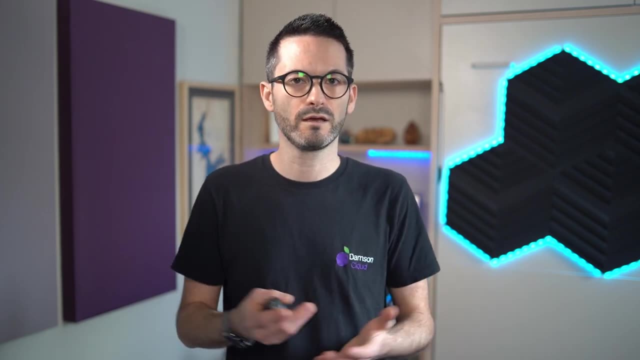 and i kind of feel here like we've seen interesting examples in in all of these different areas where you know a customer isn't using dlp but they have data loss prevention. on uh, the google workspace system, they've upgraded to enterprise but they're not actually leveraging that, those dlp or context. 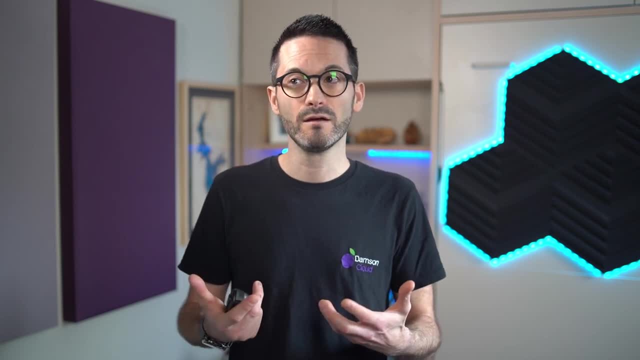 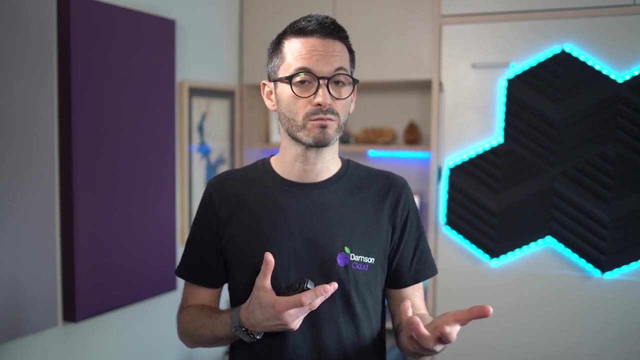 aware, access features. that's a very common one. also, we see when an organization has had google workspace for a long time, maybe some settings that were in place again when the organization was was smaller. so, for example, when you create a document that anyone in the organization can read, that 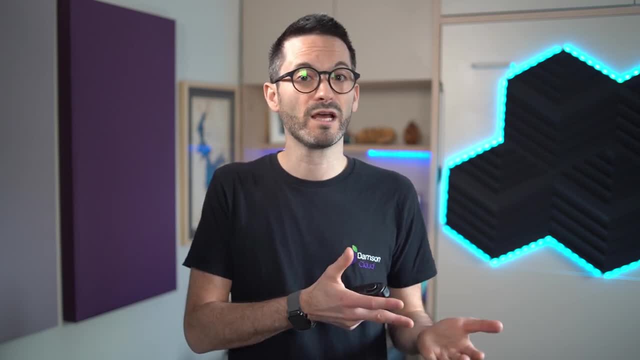 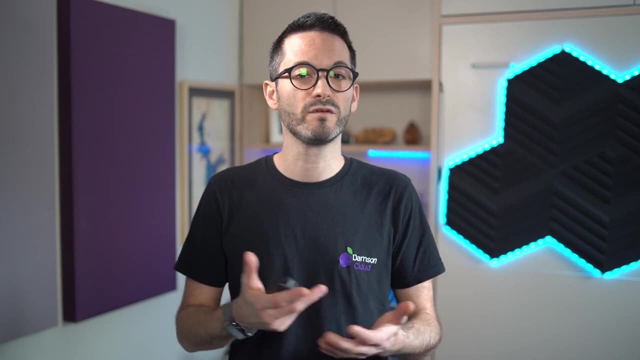 document if they have the link. now that might be fine when you're 10 users or 50 users, but when you're 100 or a thousand, you maybe you don't want everybody to be able to just view a document if they have the link. and again, people might be able to just view if they have the link, and so it's not. 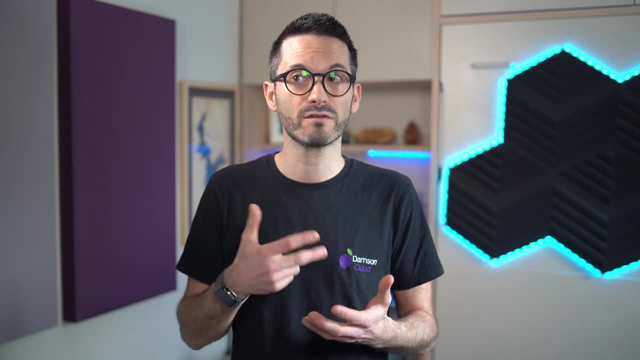 for everybody's really the final decision, but it's down to the scenario. so when you have a patient and maybe you don't want everyone to be able to just view a document if they have the link, and again people might might think, oh, that's okay, they'd have to get the link. but I've seen scenarios where maybe 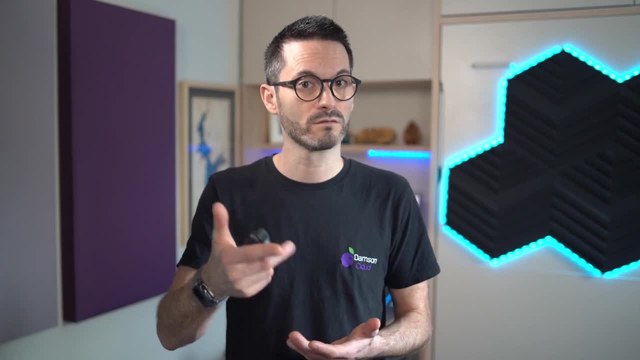 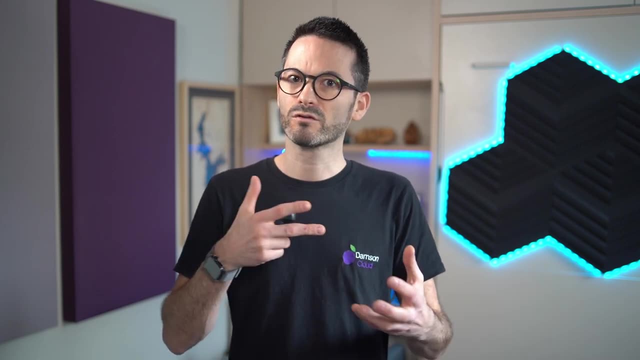 someone has put a link to a document in a calendar appointment. the calendars are set up that everybody can see everybody else's calendar- again maybe an early setting within the business- and suddenly someone has access to a document that they shouldn't. So again, it's just about. 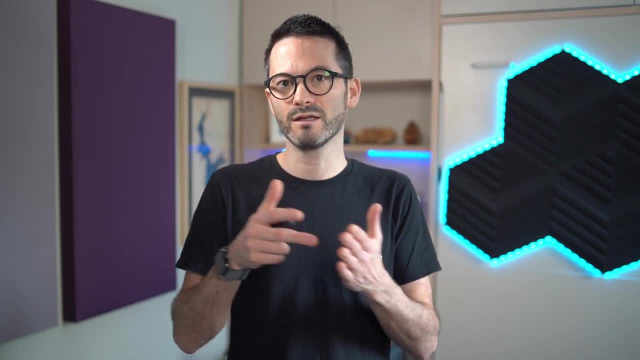 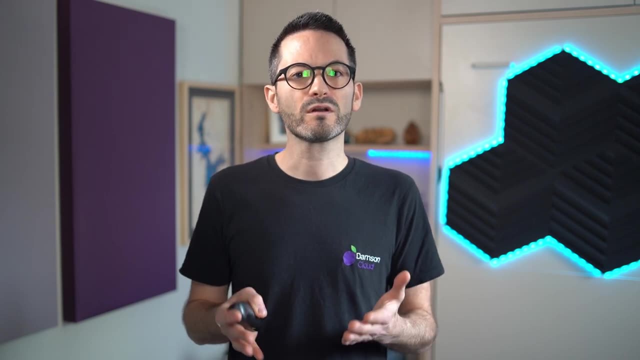 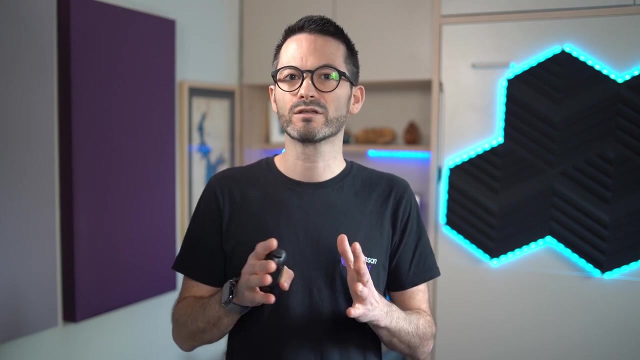 evaluating those settings, documenting them and seeing. is that the best practice, and does that make sense for us, for our organization? So what are the steps of a security workspace assessment? Well, before I go into this, I thought it might be useful to look at the scope and what we tend to. 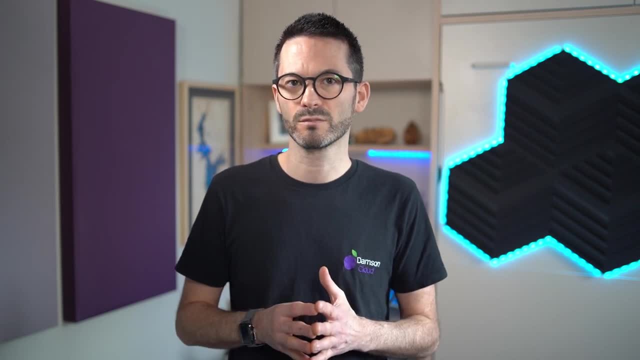 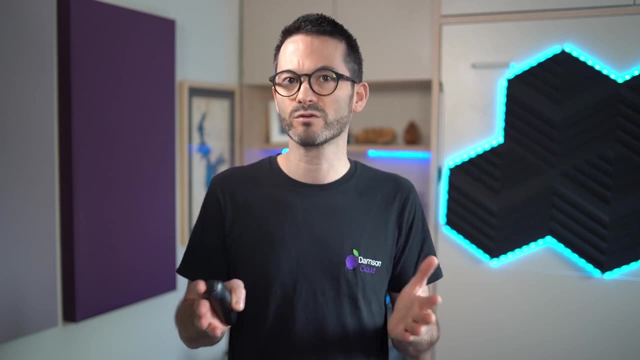 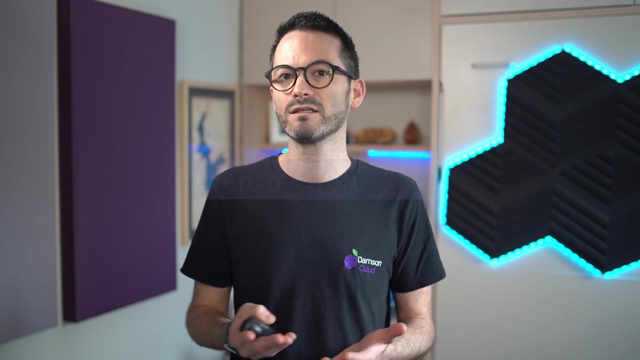 include within the scope of the security auditor assessment. The technical configuration is an obvious one. we're going to review those security configurations and processes that are associated with Google Workspace. we're going to look at the policies and procedures and the best practices that Google have, and we're going to look at things like identity and authentication. 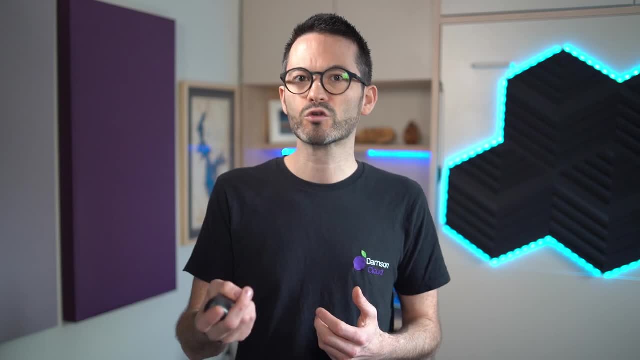 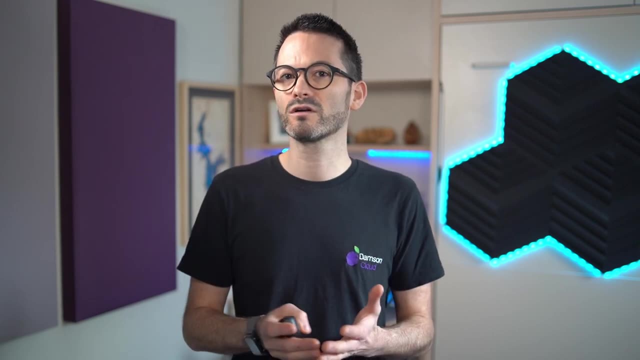 account recovery, user provisioning, you know, controlling administrator access. we often see that too many super admins on an account. we're going to look at things like e-discovery, security operations, admin alerts, event monitoring, incident response handling within Gmail. we're going to look. 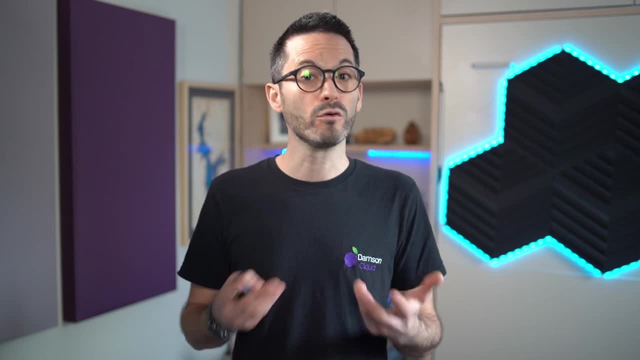 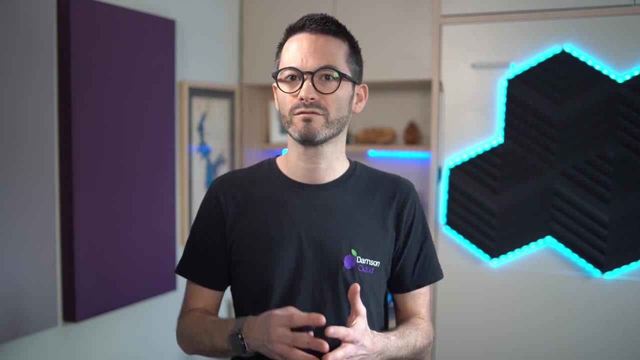 at authentication, encryption, content compliance. Google Drive is another popular area, looking at the sharing settings, the syncing capabilities, the DLP within Drive, access controls for other services like maybe Google Calendar, Google Analytics, Google Analytics, Google Analytics, Google. 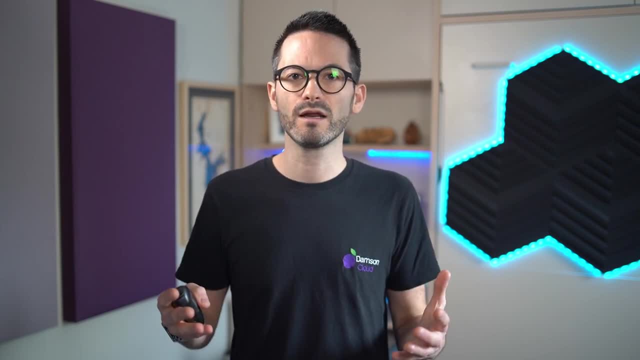 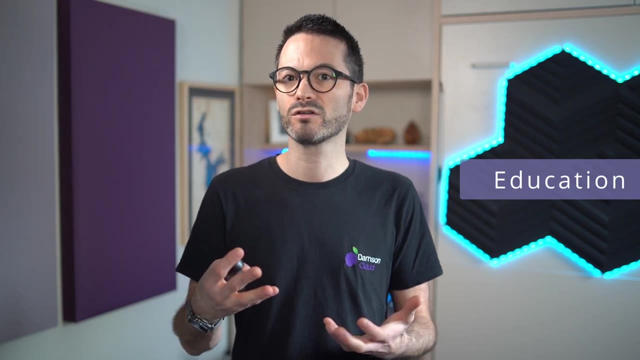 Calendar or chat or Meet directory services, and then, at kind of a high level, we're going to look at those device management capabilities. We're going to make sure that we educate your team, that we guide them on how to execute on these top priorities that we're recommending, and then 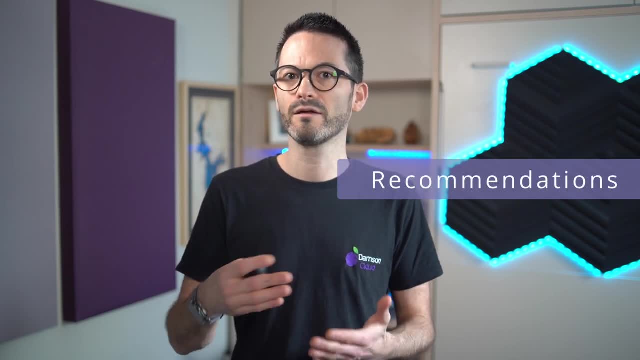 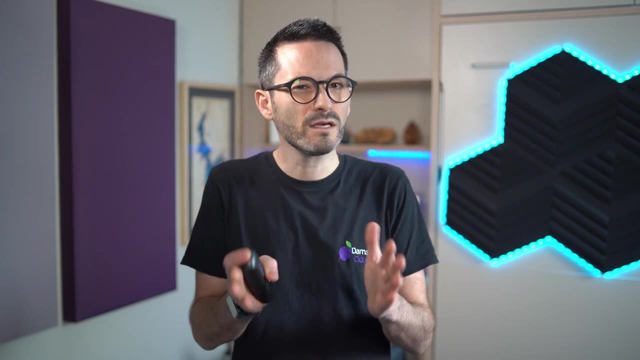 obviously we're going to give that recommendation plan and the execution plan, that with the prioritizations that your team can take away and actually execute on that. What kind of things are out of scope? So out of scope is going to be stuff like Chrome OS browser security configurations. 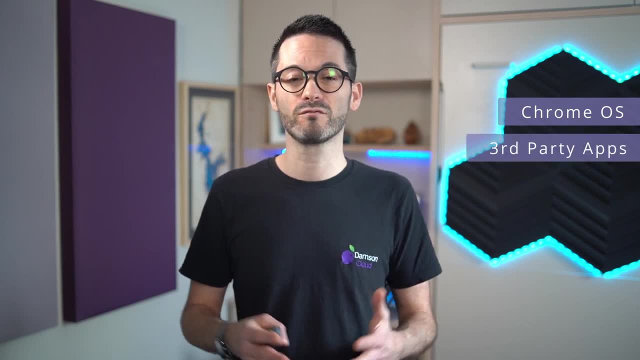 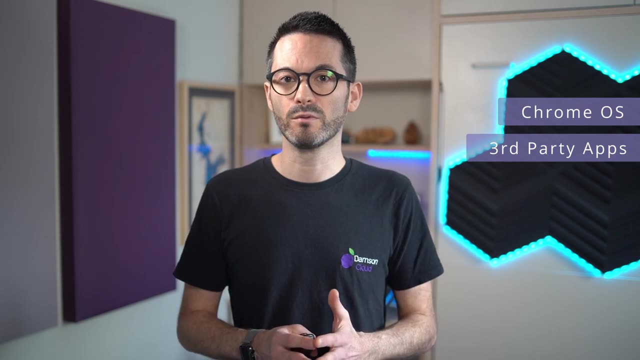 third-party apps is another big one. Customers could have dozens or even hundreds of third-party applications- We definitely don't have time to get into all of those and so they tend to be out of scope- and also the user settings within those third-party apps- Chrome web applications and the 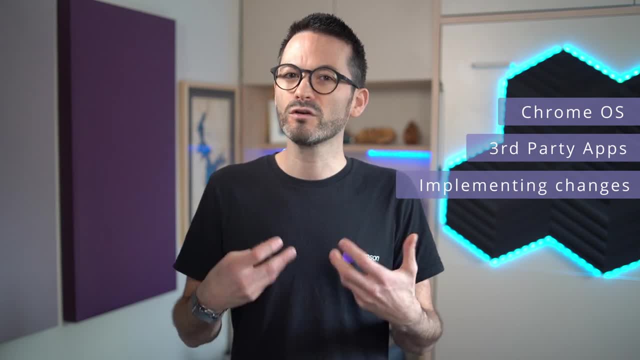 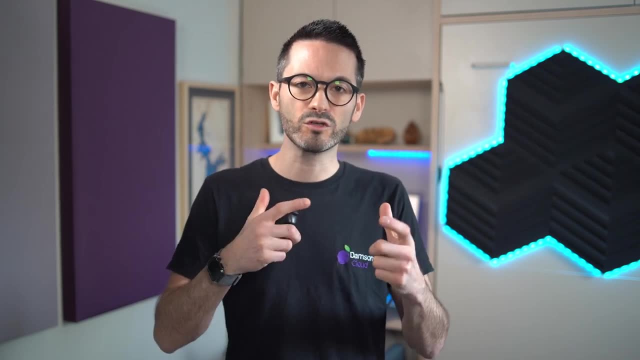 actual implementation of the changes. so the remediations, we're not going to do those as part of the audit. Sometimes customers might pay us afterwards to do those, but we generally recommend that we're doing it with the IT team because they're going to be able to do that. So 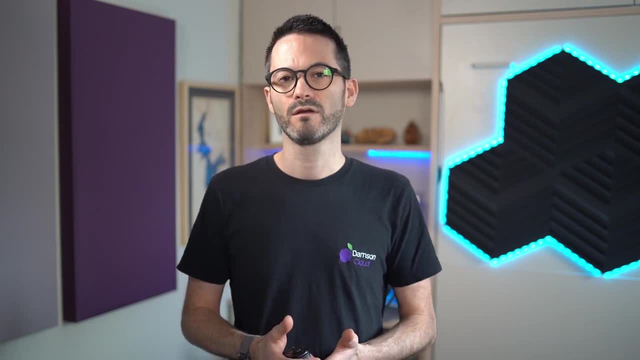 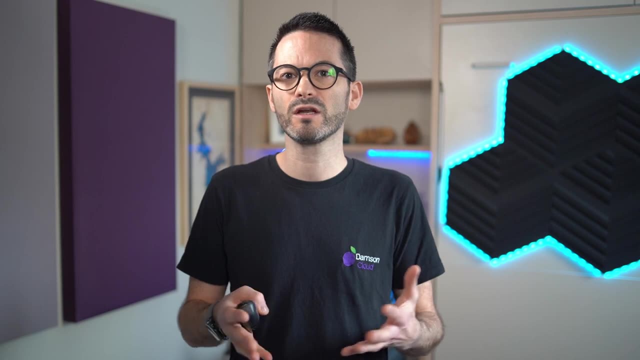 we're training and we're enabling them as part of the process. So what are the steps in the Google Workspace security assessment? Well, there's kind of four key steps. Initially, we have that kickoff meeting where we meet with the IT team and the security team and we discuss your specific 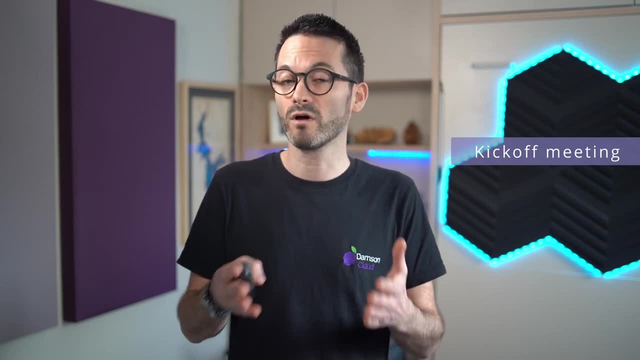 requirements. Why is it that your organization is looking to do this right now? Because that's valuable for us to know. if there's been a security incident. if it's part of an ISO audit or certification, It's valuable for our team to know if there's been a security incident. if it's part of an ISO audit or certification, It's valuable for our team to know. 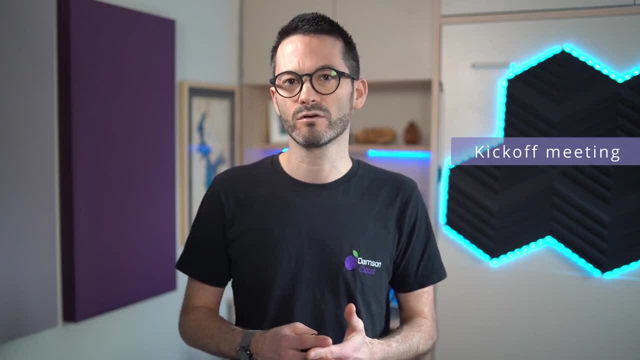 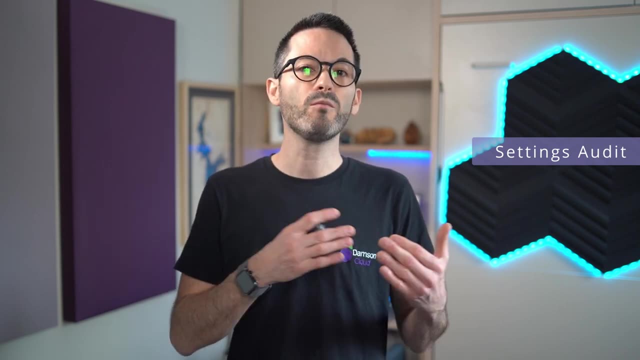 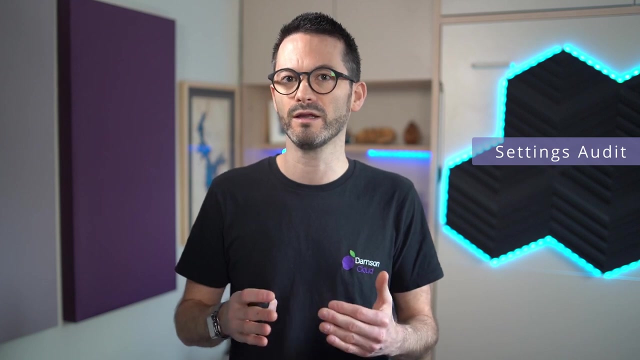 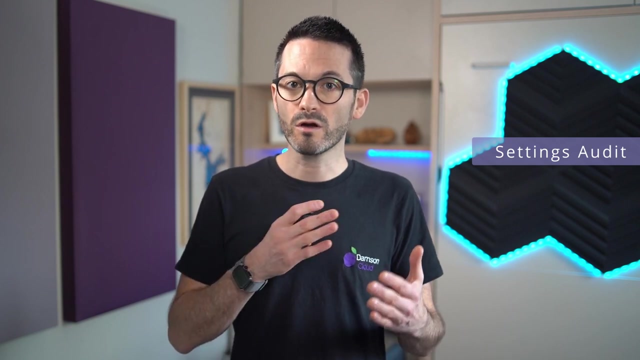 what's behind that drive to do this audit right now. Then we get administrator access. We get administrator access from you and we go and we look at the settings within your Google Workspace environment and we do that full audit and document every single feature and setting within the platform. Then we go.